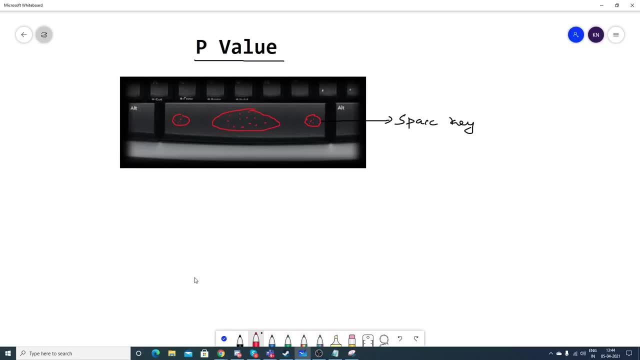 Right Now, let's do one thing. Based on this, we can definitely come up with something like this kind of bell curve. This bell curve represents one very important thing. Where there are maximum number of touches, you can see that that is the bulged part. This is how a bell curve in a normal distribution looks like. Where there are less number of touches, that is basically your tail part, And in this kind of experiment, we basically say it as two-tailed test. Okay, Because 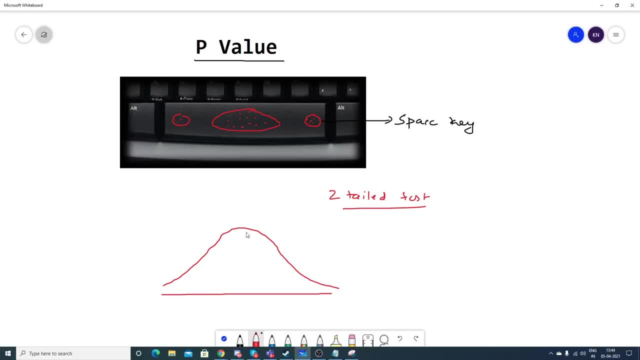 any statistical analysis we'll be doing. we'll be considering a two-tailed test which will actually provide you two specific regions on the sideways. Right Now, let me just consider that, Suppose, if I touch it over here and suppose for this particular touch, the P value is 0.01.. Now, what does this basically indicate? That we are going to understand This P is equal to 0.01 indicates that 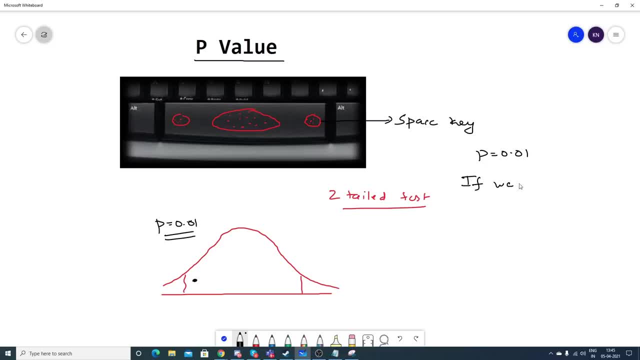 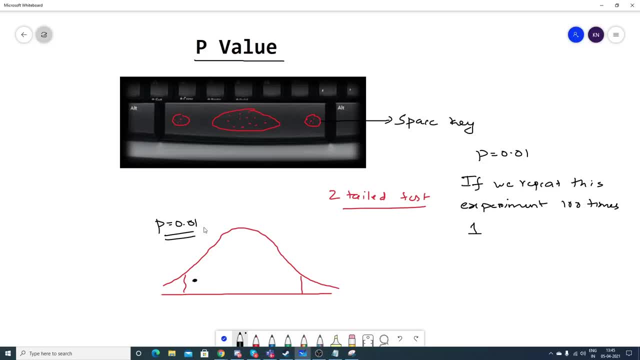 of times we will be touching this particular area will be point zero, one which is nothing but one time, one time. this is what p value basically specifies. suppose if i say that my p value over here is point eight, right, so what does this? p is equal to point eight. 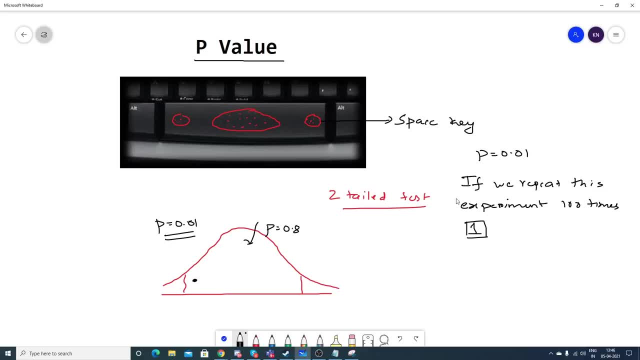 actually specify. it specifies that if we repeat this experiment hundred times, the number of times will be touching in this particular area will be somewhere around eighty times. right, that is what is the ratio that is basically given right now. let us understand and let us define. what is this p value? so, if i did, you want to define what is p value theoretical? 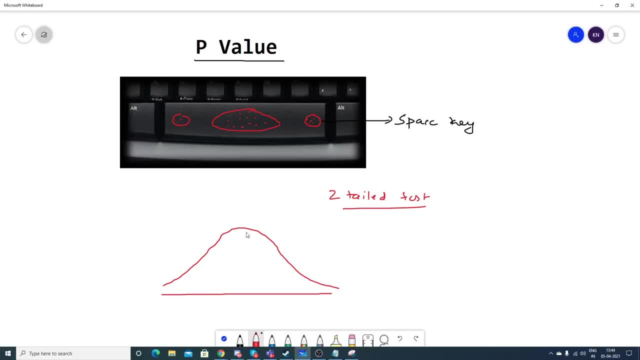 any statistical analysis we'll be doing. we'll be considering a two-tailed test which will actually provide you two specific regions on the sideways. Right Now, let me just consider that, Suppose, if I touch it over here and suppose for this particular touch, the P value is 0.01.. Now, what does this basically indicate? That we are going to understand This P is equal to 0.01 indicates that 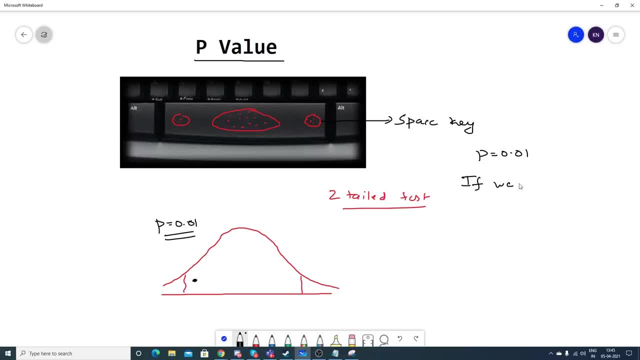 this is a neutral quarter. So, for example, say I touch the B value First, we will repeat this experiment or this experiment. If we repeat this experiment for hundred, Ne slower than that. If we repeat this experiment 100 times, then the amount of times we are going to be touching this particular area is 1.. 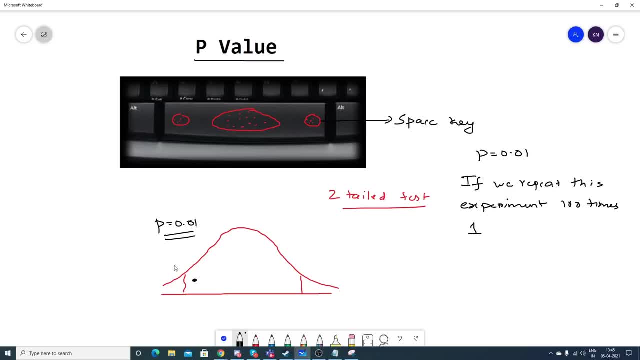 Very simple esperiment: 대 nu ti rr è lè. Very simple guys. If we repeat this experiment, which experiment? basically touching the space key Anaba? If we repeat this experiment 100 times The number of times, the number jump to the space key. 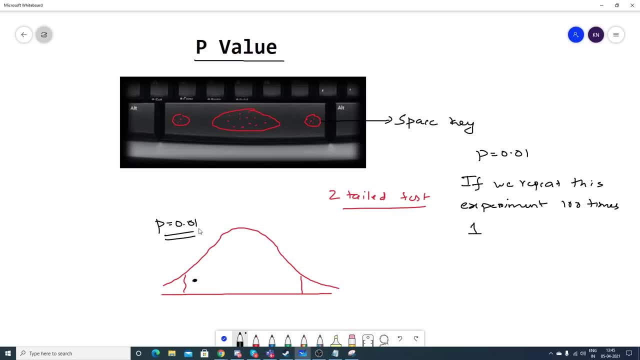 is ten times. The two terms are decentralization. This means first of times we will be touching this particular area will be point zero, one which is nothing but one time, one time. this is what p value basically specifies. suppose if i say that my p value over here is point eight, right, so what does this? p is equal to point eight. 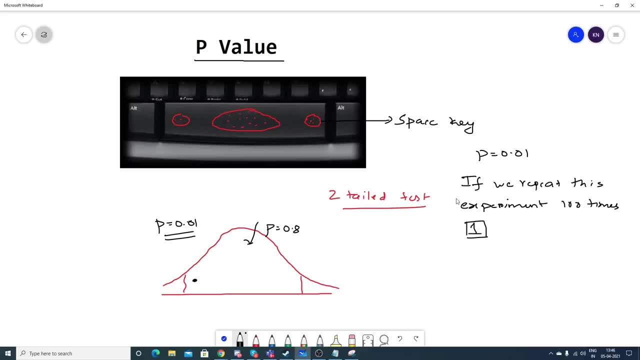 actually specify. it specifies that if we repeat this experiment hundred times, the number of times will be touching in this particular area will be somewhere around eighty times. right, that is what is the ratio is basically 1.. right now lets understand and less define. what is this p value? ok, so if i want to define, 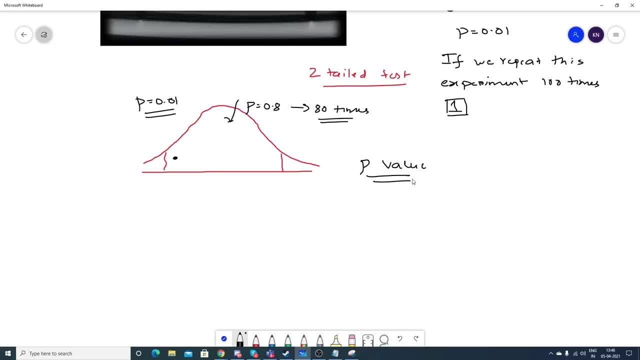 what is p value? theoretically, i can say that it is the probability. it is the probability for the null hypothesis to be true, For the null hypothesis. So, Gary, If i try again to be true, to be true, yeah, you have heard this definition, guys, it is a probability for the null. 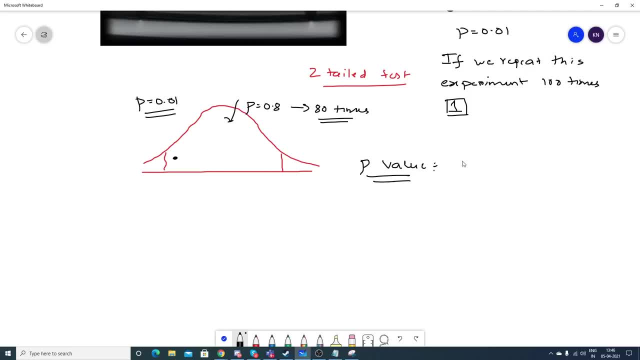 theory i can say that it is probability. it is the probability for the null hypothesis to be true, for the null hypothesis. Here what we can do is that we can dump the final relation Here u all the different values of the formula vão term l to the one i am going to define. 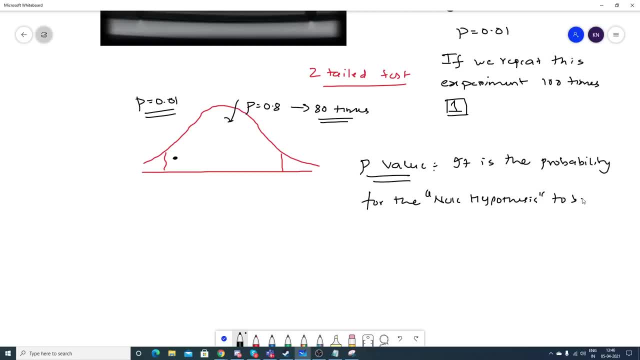 to be true. to be true. yeah, you have heard this definition, guys. it is a probability for the null hypothesis to be true. now you may be thinking: what is null hypothesis? let me define null hypothesis also for you. so i'm just going to write over here: null hypothesis. sorry for my bad handwriting, but 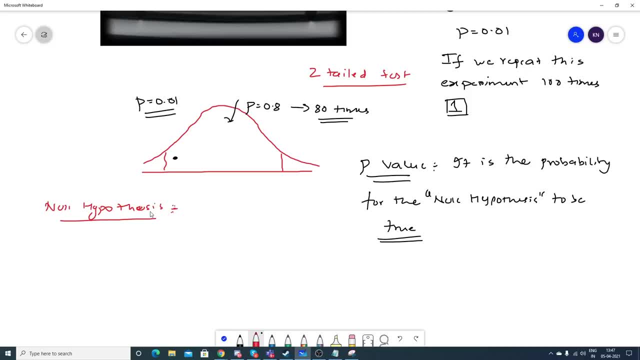 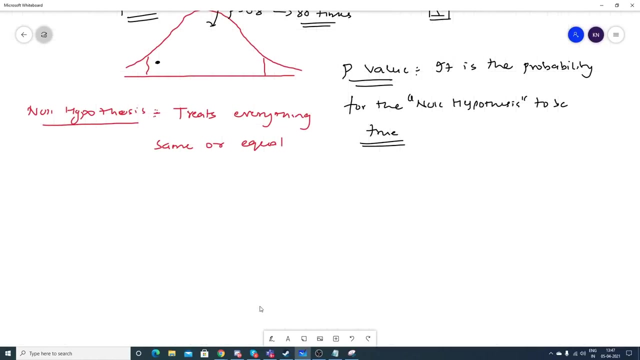 i am just trying to explain you the best possible way that i can. okay, so when we talk about null hypothesis, it treats everything same or equal. that's it: it treats everything same or equal. now let's take a very good example, a very simple example i'm going to take. consider that i want 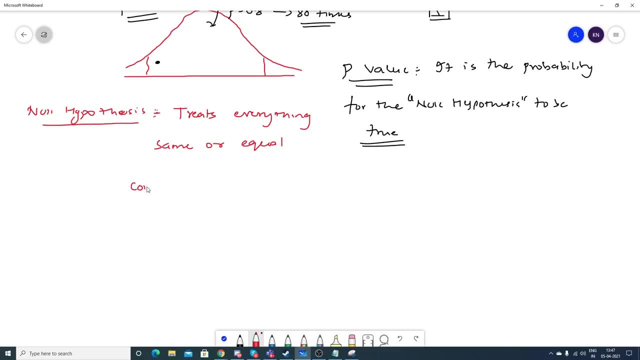 i have a coin, i have a coin, okay, and this is a fair coin, this is a fair coin. fair coin basically means that if i am performing this specific toss experiment, toss experiment, hundred times, then they, based on this fair nature, at least 50 times head should be there. right, 50 times head should be there, or 50 times tail should be. 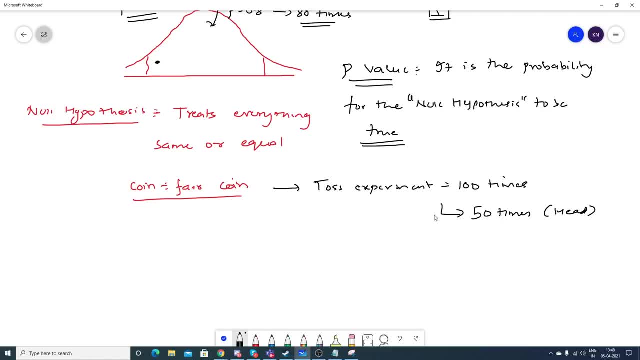 coming up right. so this is a toss experiment. okay, now, in this particular case, if i consider the null hypothesis, i'll be saying that, okay, it is a fair coin. okay, so i i may define my null hypothesis by s zero. i may say that the coin is fair. 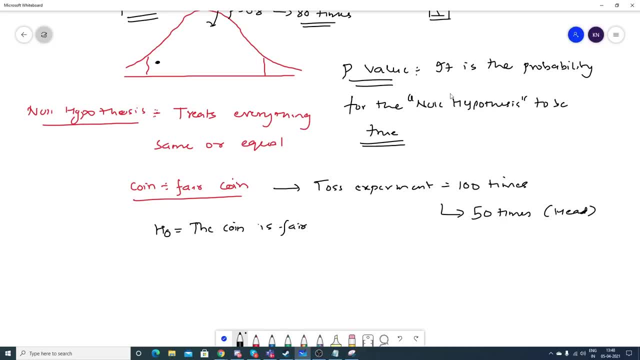 the coin is fair. okay, now see over here, guys. it says what? what is this null hypothesis? it treats everything same or equal, right, so the coin is fair. in my alternate hypothesis, it will be opposite of this. the coin is not fair, right? so i have this two information. now what i do is that i perform some kind of experiment. 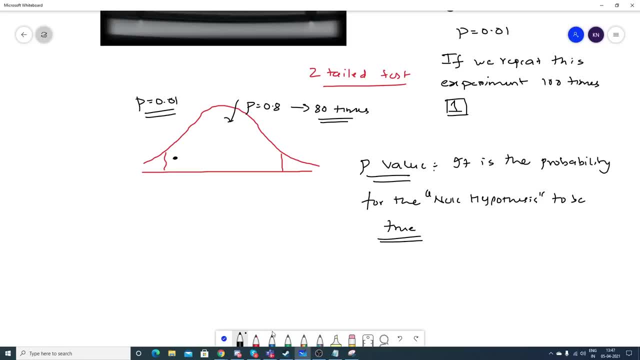 hypothesis to be true. now you may be thinking: what is null hypothesis? let me define null hypothesis also for you. so i'm just going to write over here: null hypothesis. sorry for my bad handwriting, but i am just trying to explain you the best possible way that i can. okay, so when we talk about null 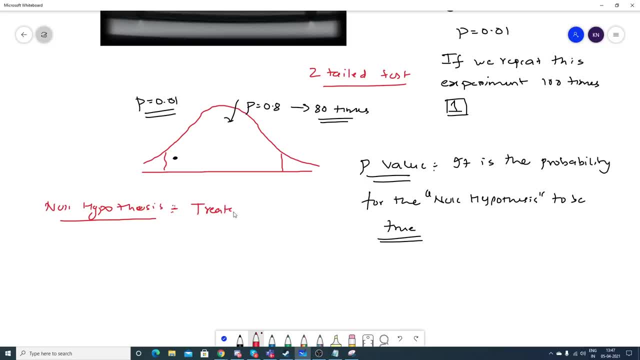 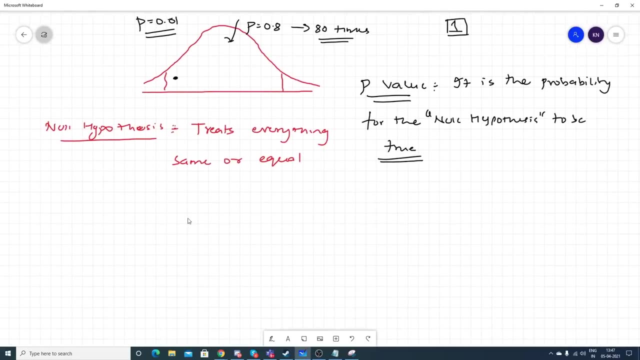 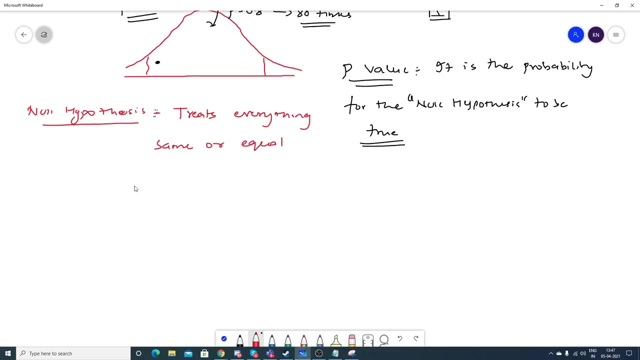 hypothesis: it treats everything same or equal. that's it: it treats everything same or equal. now let's take a very good example, a very simple example i'm going to take. consider that i want, i have a coin, i have a coin, okay, and this is a fair coin. 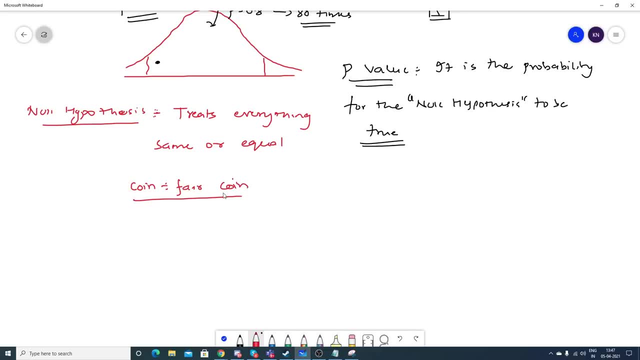 this is a fair coin. fair point basically means that if i'm performing this specific toss experiment, toss experiment, hundred times, then they, based on this fair nature, at least 50 times head should be there, right, 50 times head should be there or 50 times tail should be coming up. 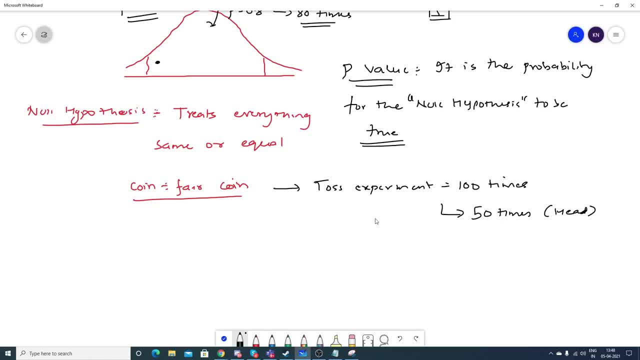 right. so this is the talks toss experiment. now, in this particular case, if i consider the null hypothesis, i'll be saying that, okay, it is a fair coin. okay, so i i may define my null hypothesis by s0. i may say that the coin is fair, the coin is fair. 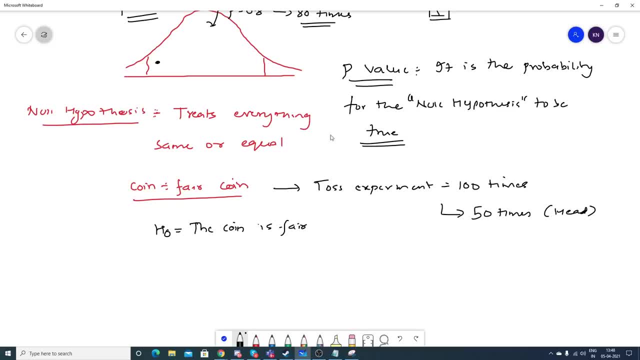 okay, now see over here, guys. it says what? what is this null hypothesis? it treats everything same or equal. right, so the coin is fair. in my alternate hypothesis, it will be opposite of this. the coin is not fair. all right, so i have this true information. now what i do is that i perform some kind of experiment. 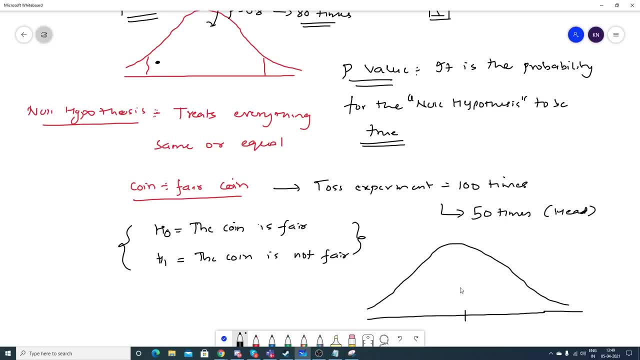 now in this experiment. we know that my mean value is 50. right, because 50 times i'll be either getting head or tail. now let me perform this particular experiment now. once i perform this experiment 100 times, i do it now. out of that, i i achieved that. i have got somewhere around 60 times. 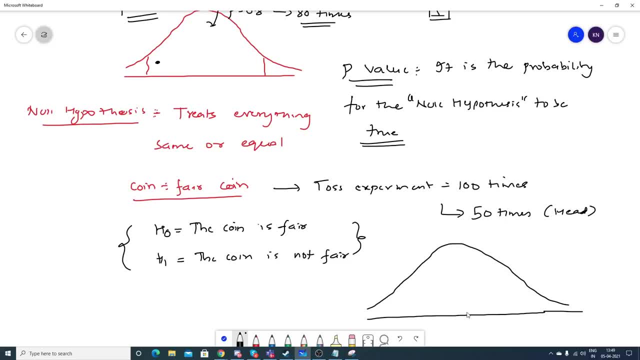 now in this experiment. we know that my mean value is 50. right, because 50 times i'll be either getting head or tail. now let me perform this particular experiment now. once i perform this experiment 100 times, i do it now. out of that, i i achieved that. i have got somewhere around 60 times. 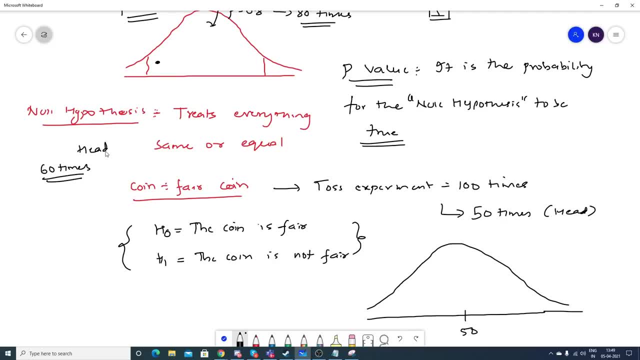 i've got head. suppose now what is 60 times over here? 60 will come somewhere over here. consider, over here 60.. now if i go and try to see this specific region, obviously i'll be able to understand that how much standard deviation away it will be from here. 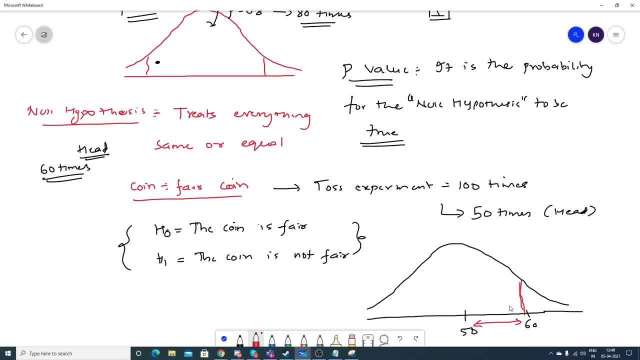 right and based on my p-value- and always remember, guys, based on this particular experiment, it is always good that we should be able to get this particular output. or is this particular experiment nearer to your mean? okay, if you get extreme to the mean, extreme right towards the mean, like this specific region, suppose, or at 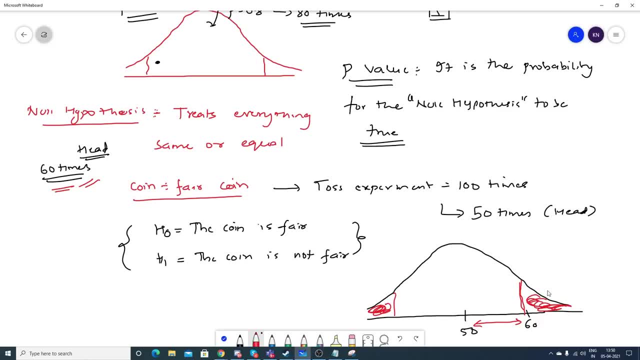 this specific region because, remember this, both are symmetrical right this region, are both symmetrical right. when this: both regions are symmetrical. obviously you can consider that this is my tail end right, as we are doing a two tail test, so this tail end will probably have your suppose. this has my 95. 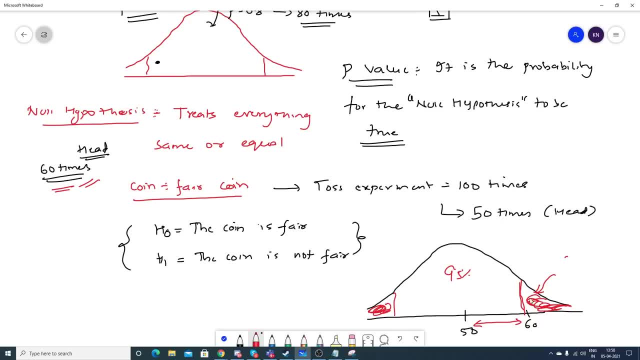 percentage of your data. this region and this probably remaining 5% will be divided as 2.5 percent and 2.5 percent. so understand, based on this particular experiment we should always try to get. if I need to make this null hypothesis as true, I really need to get all those values, or whatever experiment I am doing. 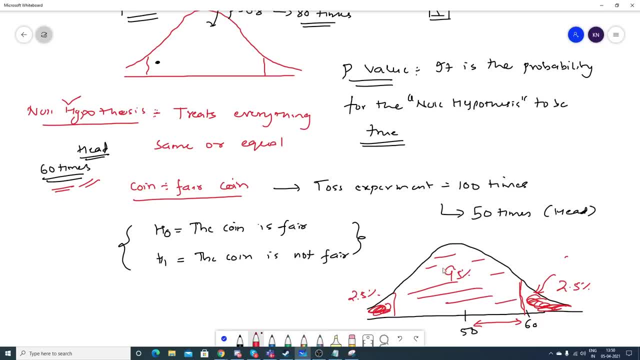 in this specific region, right, in this specific region. now, suppose, if I consider my P value as 0.05, we also say this P value as significance value, significance value. now, what does this P value see? now see with respect to 0.05? that basically. 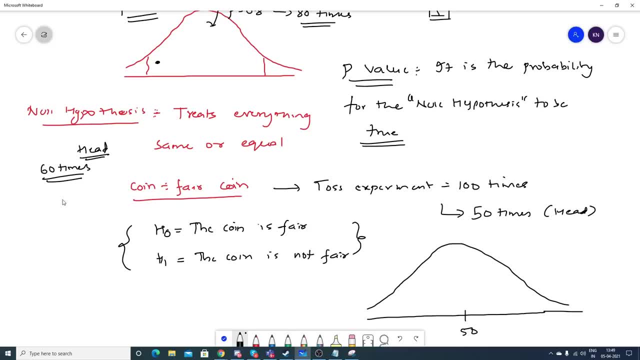 got head. suppose now what is 60 times over here? 60 will come somewhere over here. consider over here 60. now, if i go and try to see this specific region, obviously i'll be able to understand that how much standard deviation away it will be from here, right and based on my p value and 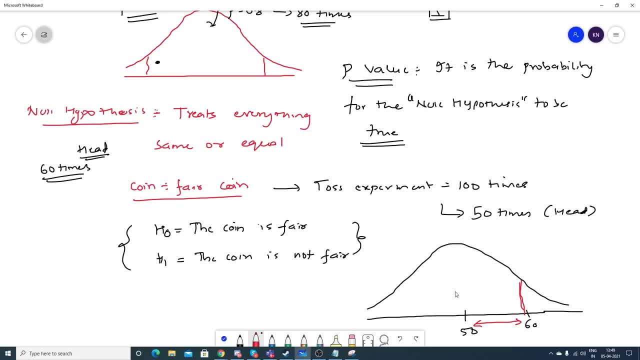 always remember, guys, based on this particular experiment, it is always good that we should be able to get this particular output, or in this particular experiment, nearer to your mean. okay, if you get extreme to the mean, extreme right towards the mean, at this specific region, suppose, or at this specific region, because, remember this, both are symmetrical- right, this regions? 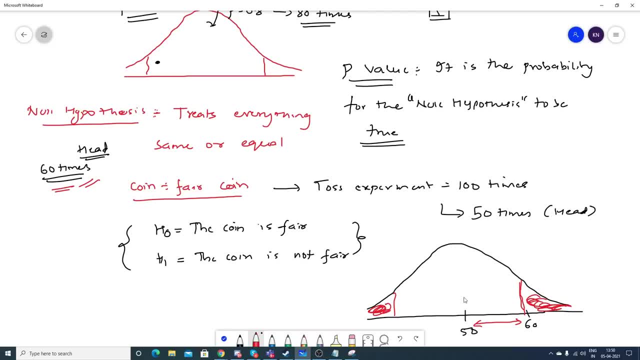 are both symmetrical, right when this, both regions are symmetrical. obviously, you can consider that this is my tail end, right, as we are doing a two tailed test. So this tail end will probably have your- or suppose this has my- 95 percentage of your data. this region and this probably remaining 5 percent will be divided as 2.5. 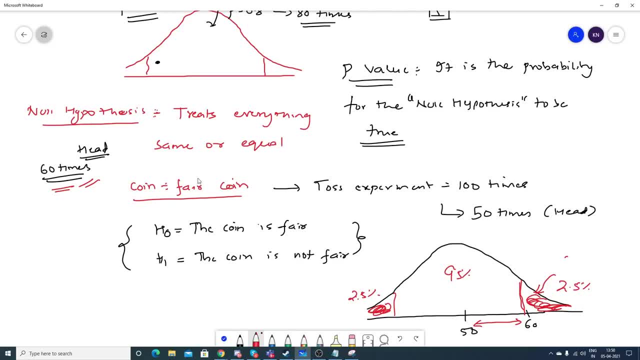 percent and 2.5 percent. So understand, based on this particular experiment we should always try to get. if I need to make this null hypothesis as true, I really need to get all those values or whatever experiment I am doing in this specific region right in this specific region. 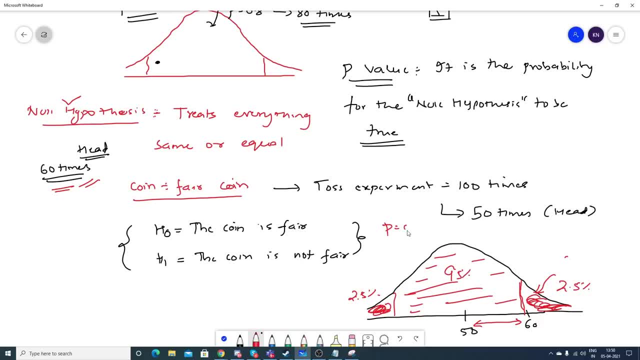 Now suppose, if I consider my p value as 0.05, we also say this p value as significance value, significance value. Now, what does this p value say? Now see, with respect to 0.05? that basically means says 2.5 percentage of data at this side and 2.5 percentage of data at. 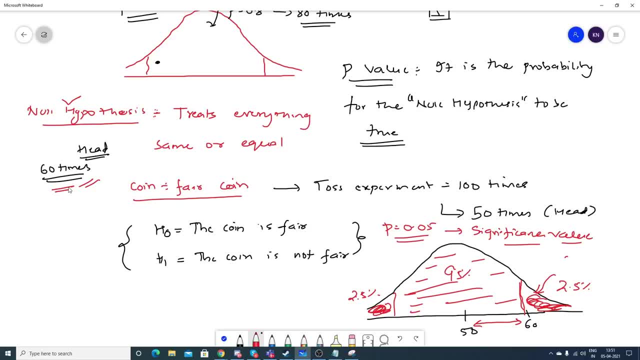 this side. If my experiment comes up with a value and if that particular value falls in this region, then I am definitely going to reject the null hypothesis. saying that, saying that, saying that over here you can see that the coin is not fair, the coin toss is not fair because 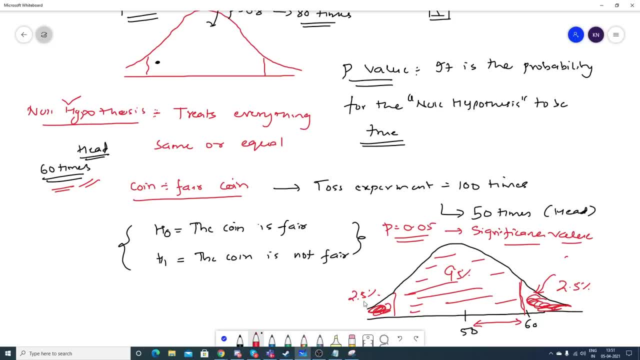 means says 2.5 percentage of data at this side and 2.5 percentage of data at this side. if my experiment up with a value and if that particular value falls in this region, then i am definitely going to reject the null hypothesis. saying that, saying that, saying that over here you can see that the coin is. 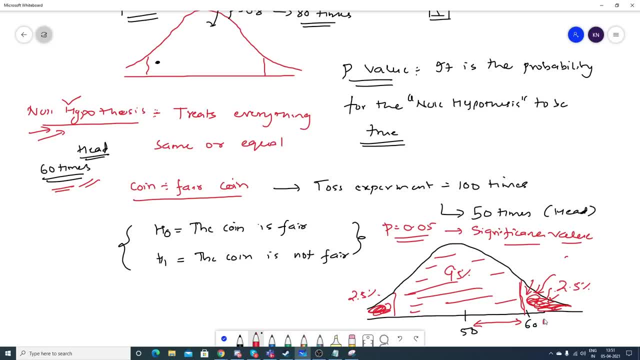 not fair. the coin toss is not fair because i'm getting a value which is very, very much far away from the mean value. now suppose, guys, i perform an experiment over here and suppose my domain expert person has told that, okay, i have to take this p value as 0.05. okay, this is. 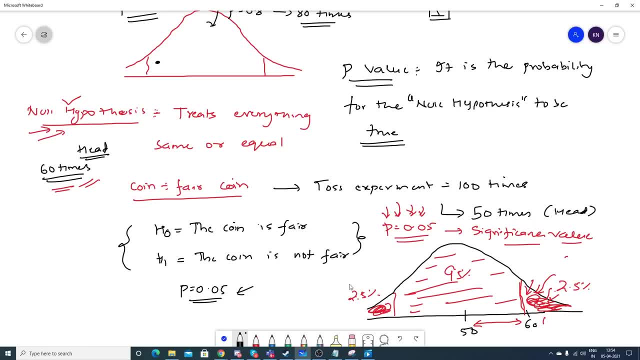 basically our tail region, which i am actually dividing based on 2.5 percent, and 2.5 percent, they have told it okay, and usually this significance- we also say this as a significance value, right, and this significance values are derived by the domain expertise, person. yes, you. 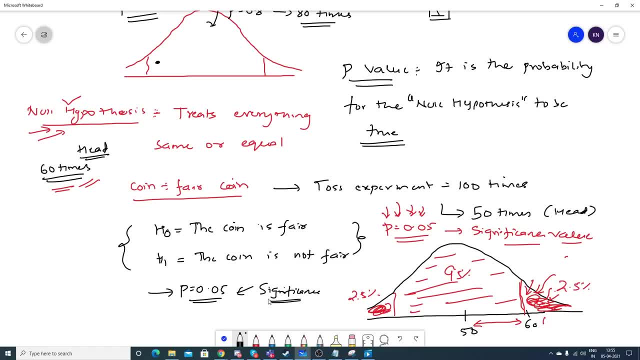 can take it as point one, zero. point two, zero. you can take out any values itself. now suppose if i perform an experiment over here and say that the coin toss is very much far away from the mean value, then i can take it as 0.05, and so the coin toss does not necessarily win over the main value. 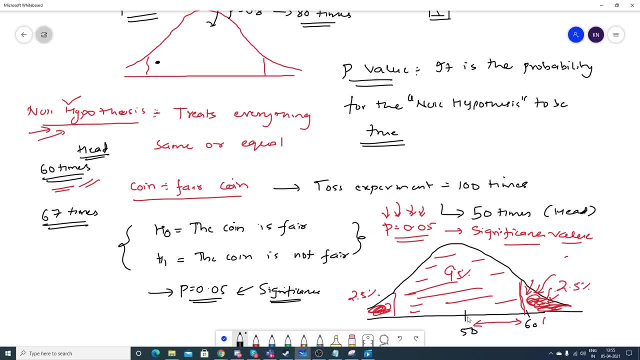 okay, so let's take an experiment where i have now got 67 times head. okay, now i'll just try to, you know, put this particular value, probably plot this particular value with respect to 67. it will come somewhere here and we know that our region of 2.5 percent is from here now. you can definitely see. 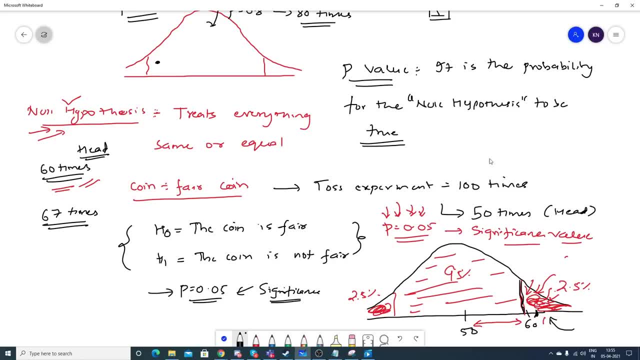 that it is falling at this specific region. now, when we see that, okay, it is falling in this tail tail region, in short, we can definitely say that right. that basically means our new experiment data that is falling. it is falling away from the mean and it is so much extreme, is so much extreme. i really need to reject the null hypothesis. 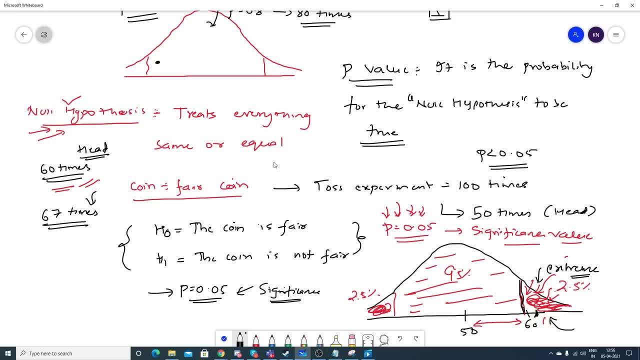 and we cannot treat everything is same or equal right. so in this particular case, null hypothesis will be. that which is fair coin will get rejected and we will come to a conclusion that this is not a fair coin. similarly, if i perform an experiment, suppose i get somewhere. 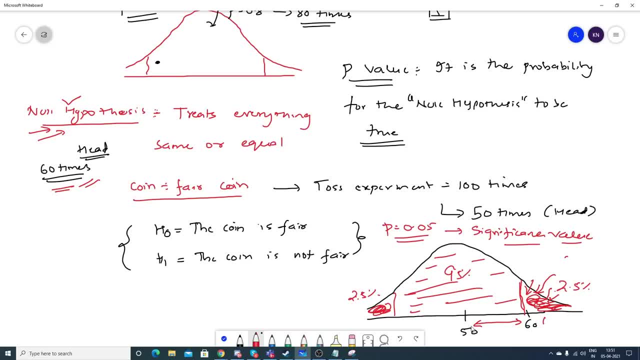 I am getting a value which is very, very much far away from the mean value. Now suppose I perform an experiment over here and suppose my domain expert person has told that, okay, I have to take this p value as 0.05. okay, this is basically our tail region, which I am actually. 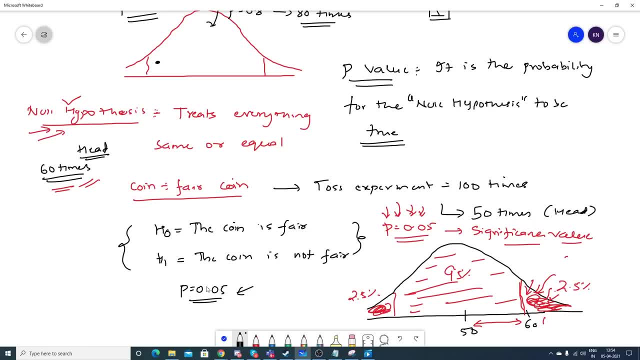 dividing based on 2.5 percent, and 2.5 percent, they have told it okay, and usually the significance- we also say this as a significance value. right, and this significance values are derived by the domain expertise person. Yes, you can take it as 0.10, 0.20. you can take it as 0.70. 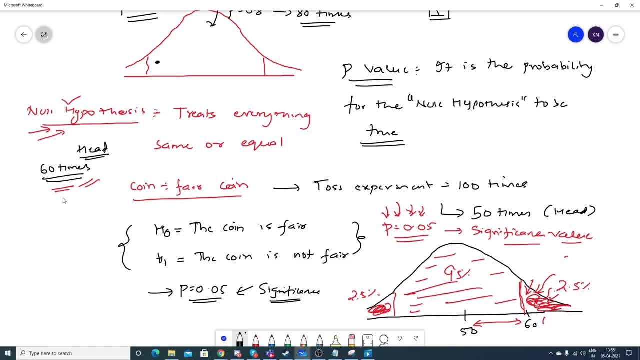 take out any values itself. now suppose, if i perform an experiment where i have now got 67 times head, okay, now i'll just try to, you know, put this particular value, probably plot this particular value with respect to 67. it will come somewhere here and we know that our region of 2.5. 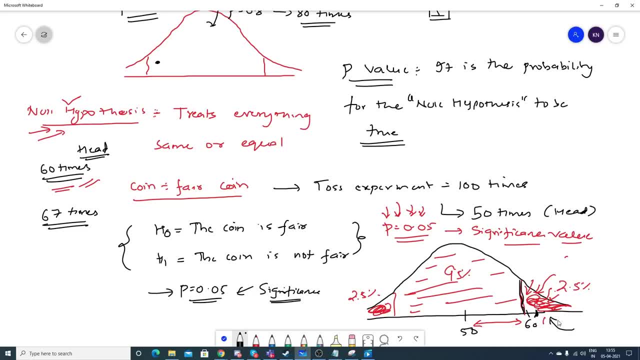 is from here. now, you can definitely see that it is falling at this specific region. now, when we see that, okay, it is falling in this tail region, in short, we can definitely say that our p value is less than 0.05. right, that basically means our new experiment data: that is falling, it is falling. 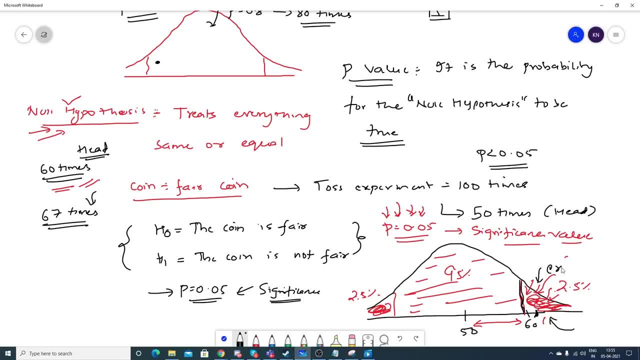 away from the mean, and it is so much extreme, so much extreme- i really need to reject the null hypothesis and we cannot treat everything is same or equal right. so in this particular case, null hypothesis will be the that which is fair coin will get rejected and we will come to a conclusion that this is not a fair 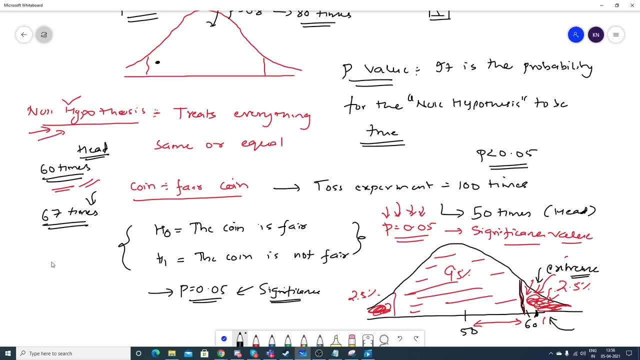 coin. similarly, if i perform an experiment, suppose i get somewhere around. you know, if i, if i just take an example of 40 times head instead of 40 times, i'll make it at 30 times head from this experiment, then again, if i try to plot it over here, it may come somewhere over here. 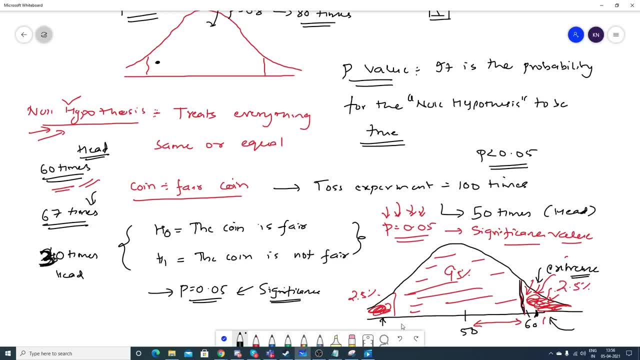 okay, and again, based on the p value, we can also derive this: how much standard deviation will be away from this and that? for that you, we usually use something called a z test, t test and all. there is also something called a z table. we, we watch that z table and we basically do it. now, when this